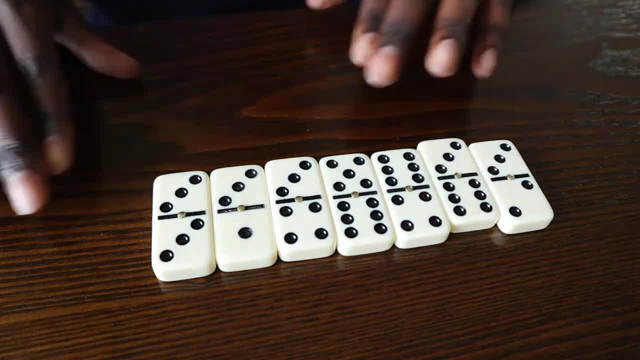 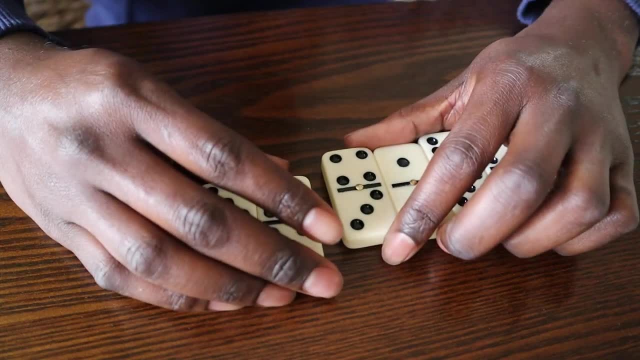 Something I always do is set my hand up for action. Ask yourself these questions when setting up your hand. Do I have a block hand? Do I have any missing suits? What is my dominant suit? Does it include a double? If it's your down, that can help you. 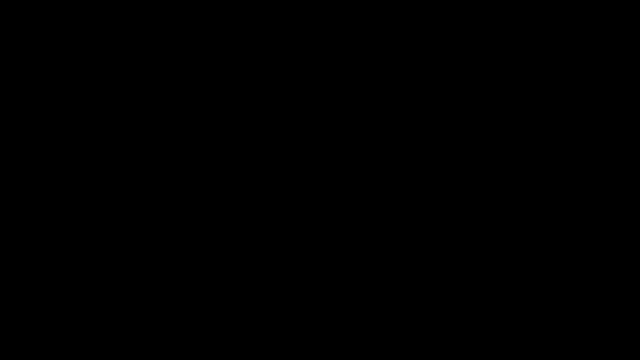 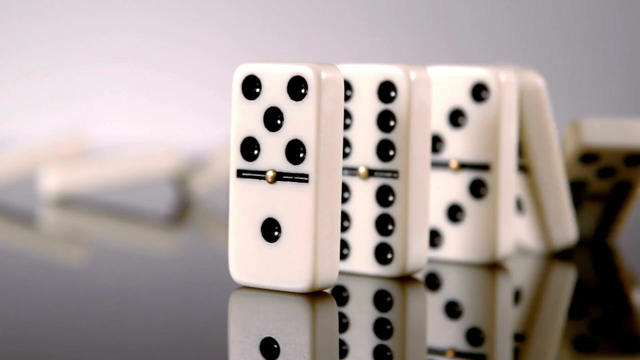 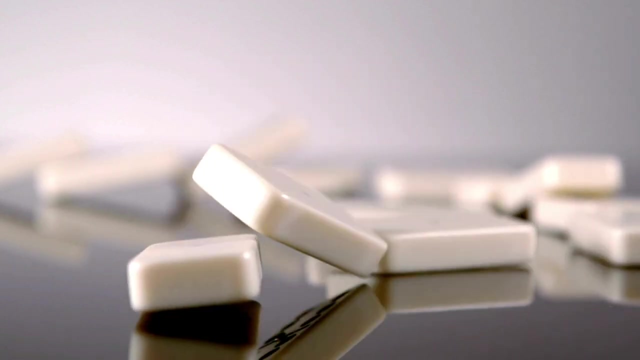 easily dictate your first play. Tip number four: drop those doubles like they're hot. Doubles can easily get locked in your hand if you don't get off them early, Since they aren't as versatile doubles such as double six, double five or double four. 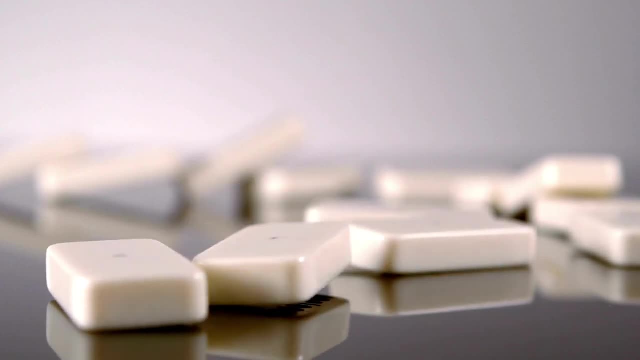 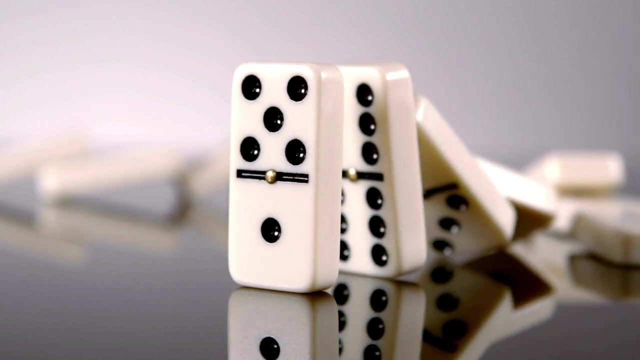 won't have as many opportunities to be played, So play them early in the hand. Of course, be mindful where you are in the stream of the game, how many points you or your opponent needs to win. If you're right at the finish line, sometimes a domino principle like drop your. 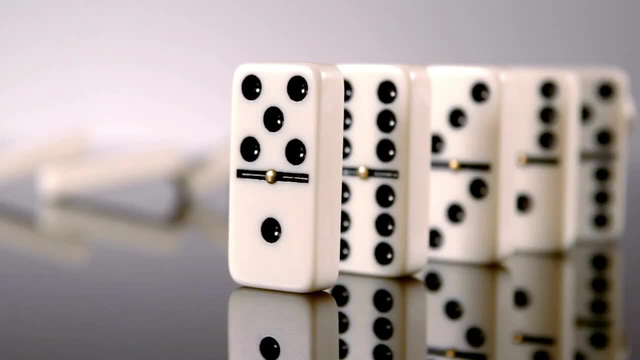 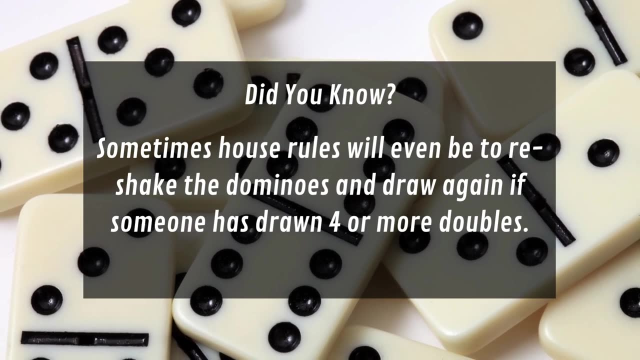 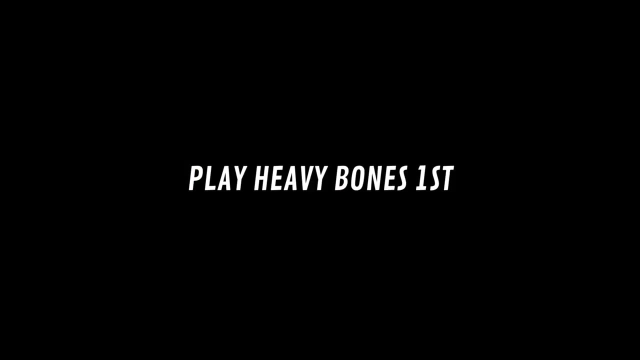 doubles early might go out the window, but it's a judgment call. Did you know? Sometimes house rules will even be to reshape the dominoes and draw again if someone has drawn four more doubles, tip number five: play your heaviest bones first. similar to the last. 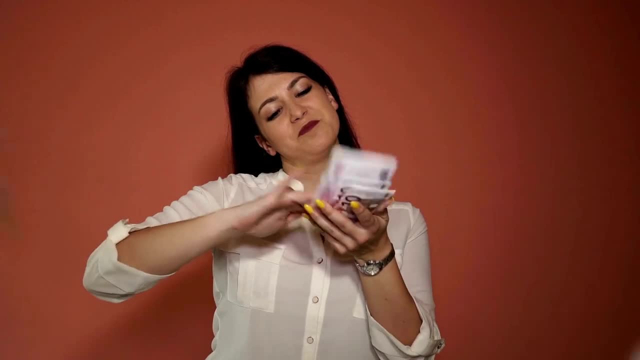 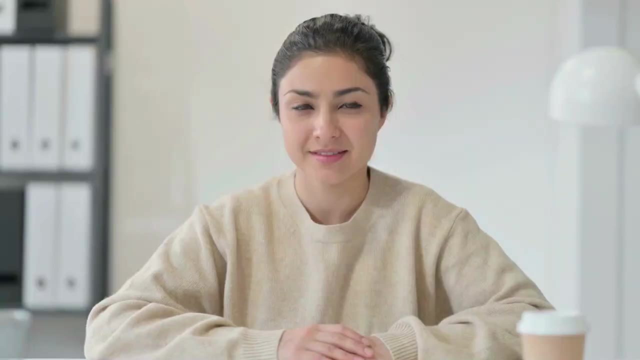 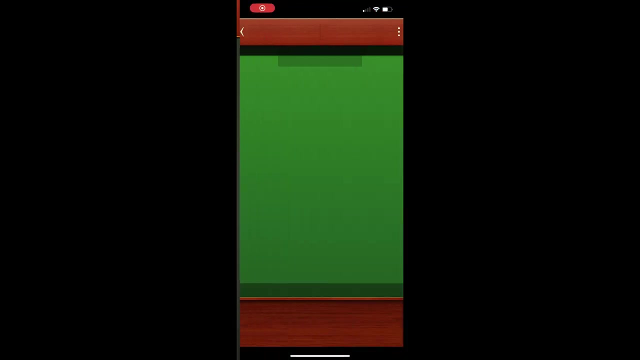 tip: playing your heavy bones first is important to avoid getting them stuck in your hand and paying them out to your opponent if they domino. if you enjoyed this video so far, please hit that like button and subscribe to the channel. so how can we apply some of the tips that we learned in this video? so I'm gonna 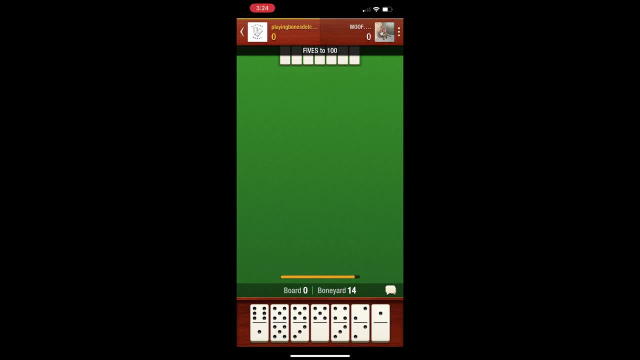 log into my fly Klopp's account and I'm gonna demonstrate exactly how to do some of the things that we talked about. so in this particular game, I'm getting to play first with double five, now, right here. this is a key moment because I could play blank one and score, but I'm not. I'm gonna go ace six. I'm playing my heavier. 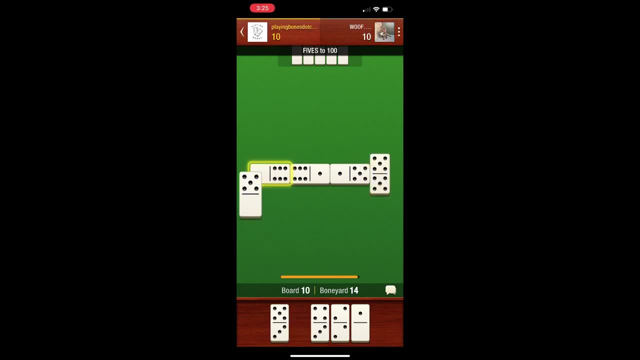 bone first. and look at that, my count is still gonna come around. I'm gonna take 15 points right here. my opponent is definitely going slow, so he's taking his time. you see, here I'm using my double. another a point applied from the video, dropping my double first.